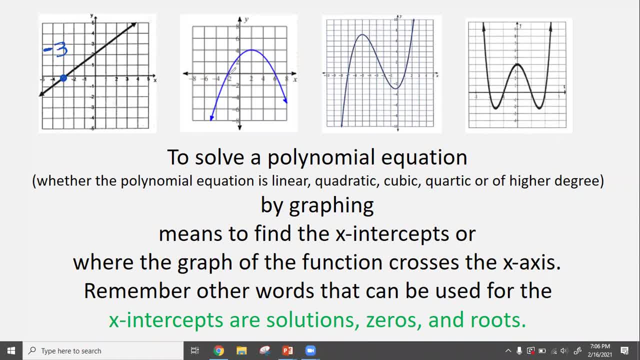 which is the graph. The graph of a quadratic is a parabola and this has two x-intercepts and they are at negative 2 and 6.. This function is a cubic and we have three x-intercepts, So the x-intercepts are at negative 7,, negative 2, and positive 1.. 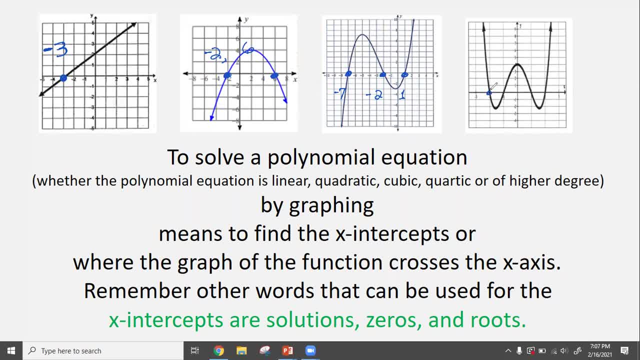 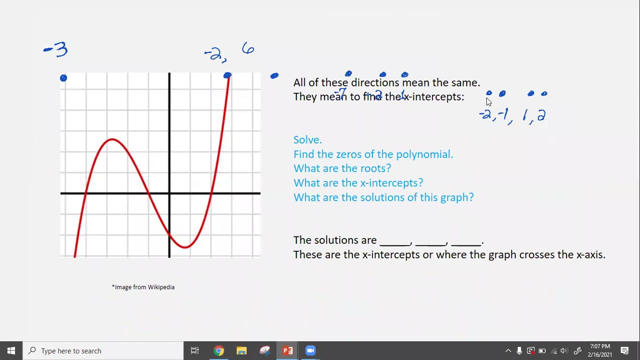 And then this quartic has four x-intercepts and they are at negative 2, negative 1, 1, 1, and 2.. Now all of these directions mean the same and mean to find the x-intercepts. So if i say solve, or i say 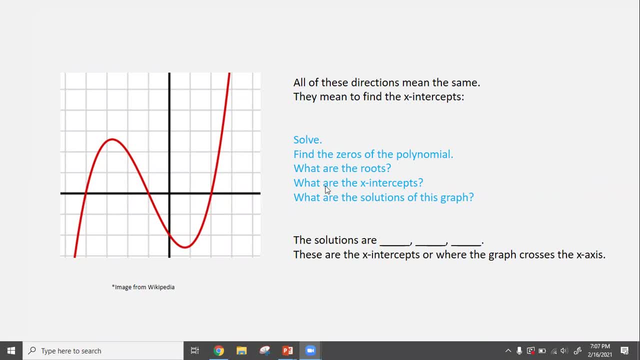 find the zeros of the polynomial. what are the roots? what are the x-intercepts? what are the solutions? the x-intercepts, the x-intercepts, the x-intercepts. what are the solutions of the graph? They all mean to find the x-axis or where the graph crosses. 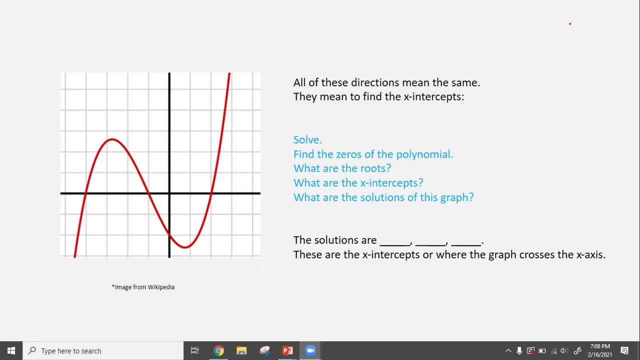 I mean the x-intercepts or where the graph crosses the x-axis. So we have three places that this graph crosses the x-axis. They are at negative one, negative, two, negative, three, negative four, negative one and positive two. 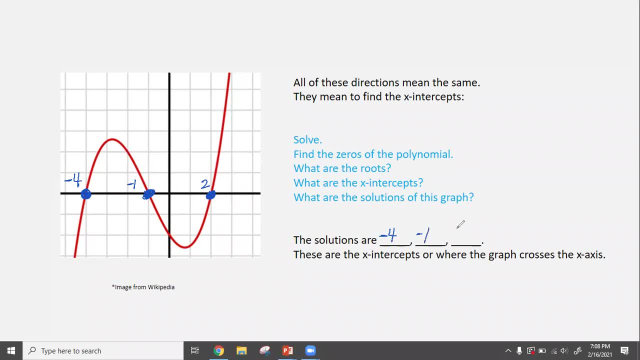 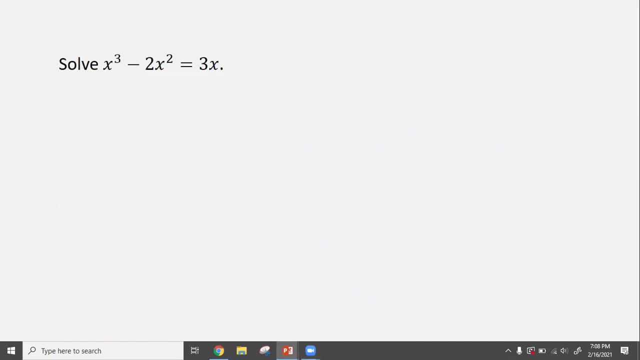 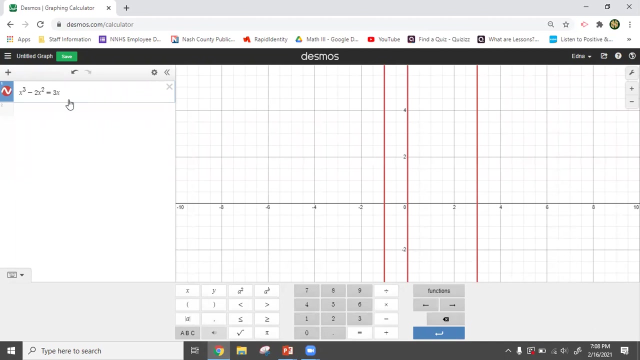 So negative four, negative one and positive two are the solutions to that graph. So what if we're given an equation without a graph? Then we use the help of decimals, And I have already placed the equation into decimals. We do not have 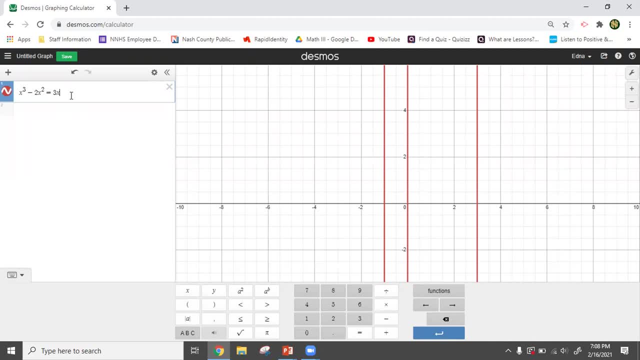 to put it equal to zero. Decimals can handle the equation just like it is, And so I placed this equation in decimals. and then I look at the x-intercepts. So here I have an x-intercept and here I have an x-intercept. 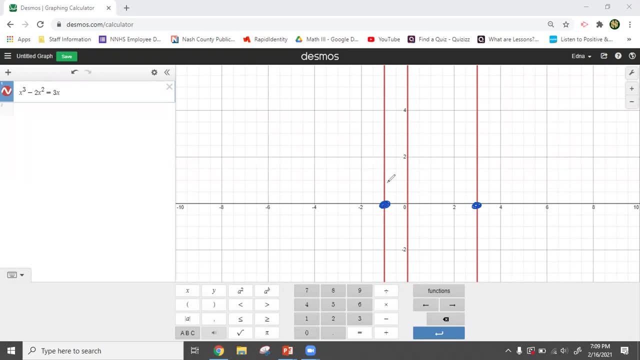 Okay, so it looks like here I'm at negative one and here I am at positive three, So I'm going to take a look at the x-intercept. I'm going to talk about the x-intercepts a little bit more because of the way it's spaced out. 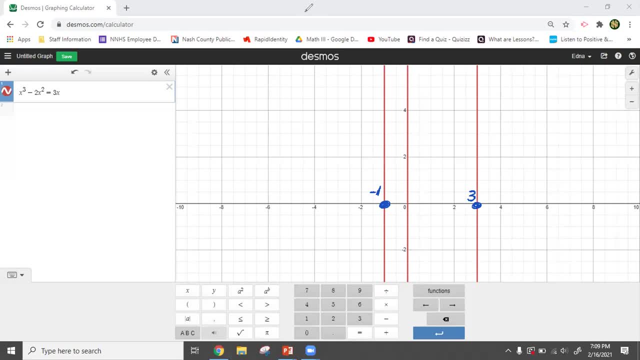 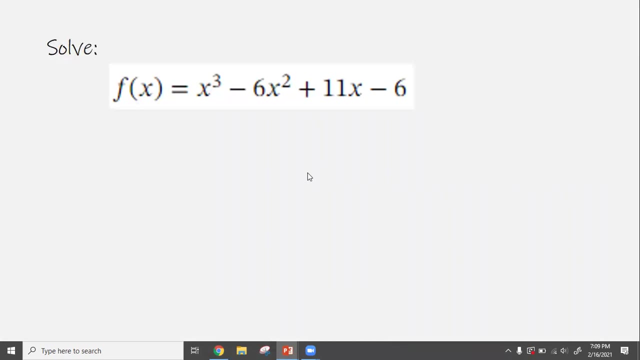 Because of the way it's spaced out. you can zoom in or zoom out if that helps for you to see the x-intercepts more clearly. So I'm going to pause the video. So I'm going to pause the video. to pause, and let you take a moment to solve this by graphing, by you placing it in Desmos. 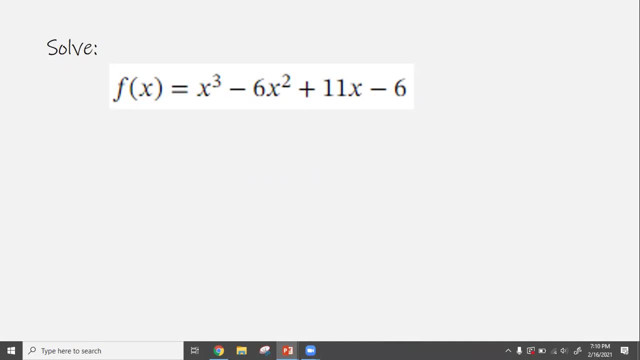 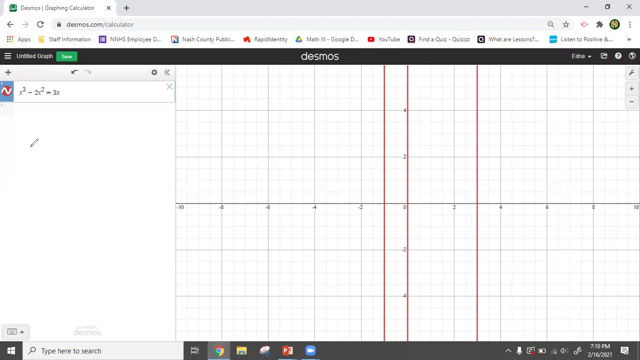 and then I'll resume and do the problem with you. Okay, so we have x to the third minus 6x squared plus 11x minus 6.. So we have x cubed minus 6x squared plus 11x minus 6, and that was equal to. 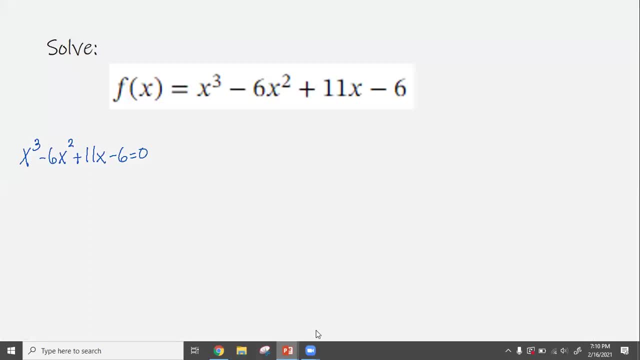 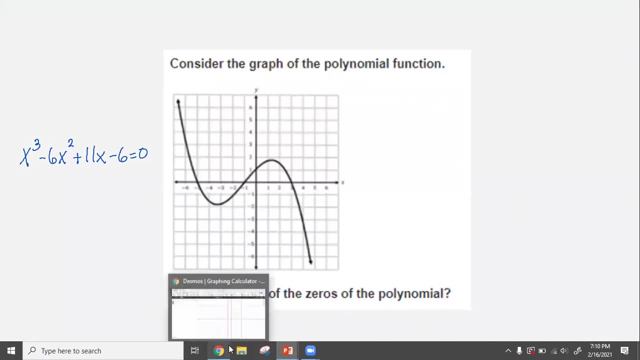 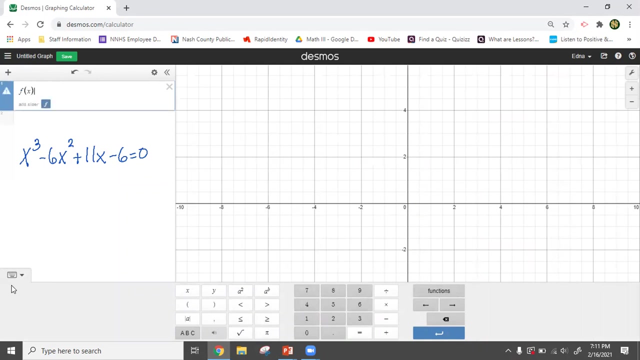 zero. Let me check Now. that was equal to f of x. So we can put it equal to zero, or we can put the f of x. It will handle that as well. So x to the third power. that's how I get to the third power minus 6x squared. 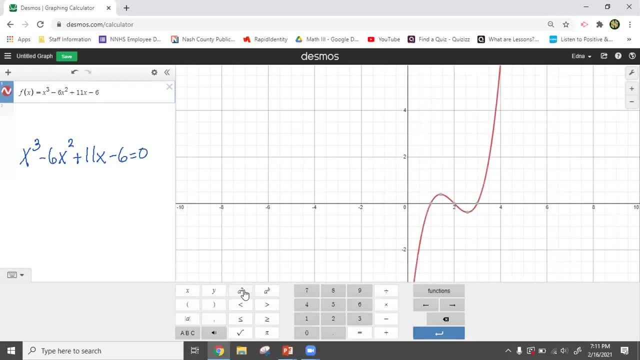 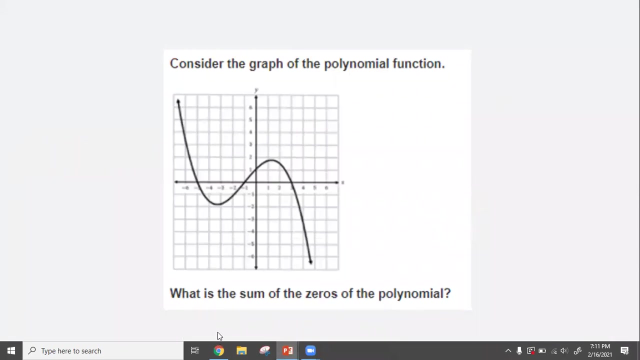 plus 11x minus 6.. So I have three x-intercepts. I have one, two and three. Now let's consider this graph Um, because this one not only wants you to find the x-intercepts, but it wants you to take the